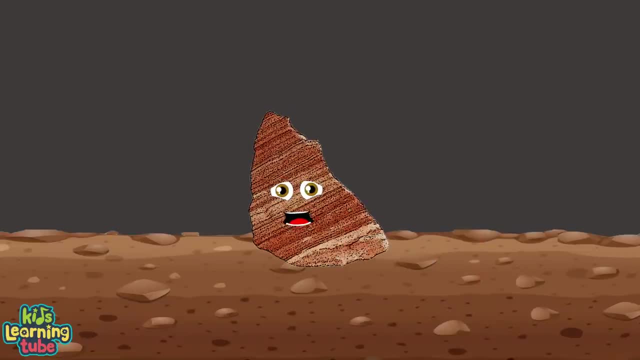 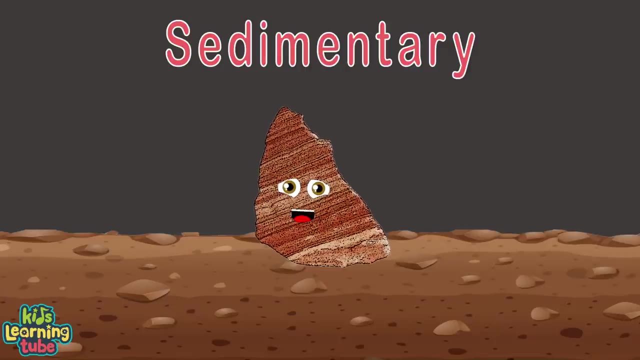 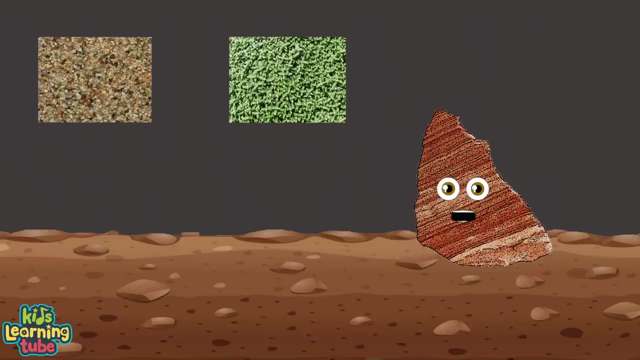 This says It's been time well spent. I'm a type of rock called sedimentary. Let's break down the meaning of my name to learn about me. Sediment's small particles of sand or organic material that settle at the bottom of water or land as gravity pulls. 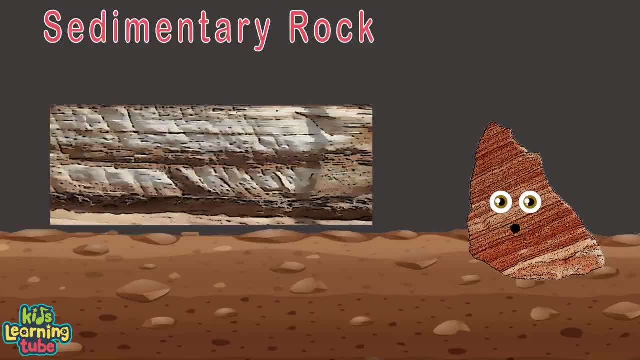 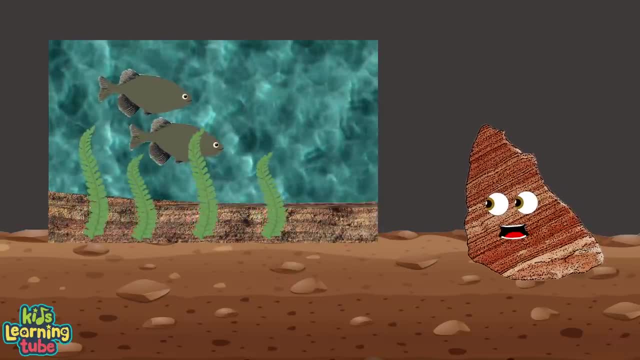 Sedimentary rock forms. when sediment builds up over time, It's compressed into layers forming rocks till they're prime. You can find lots of fossils in sediment- Sedimentary rock when plant and animal remains are squishing layers in which we had just talked. 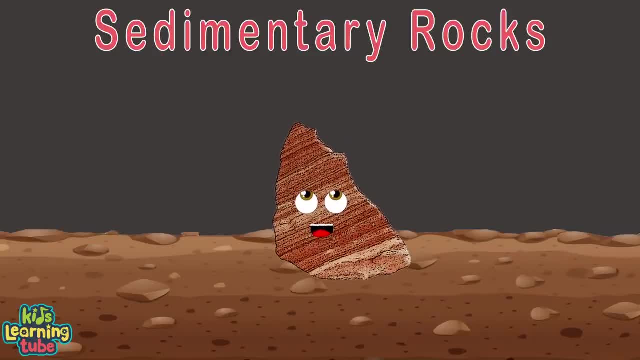 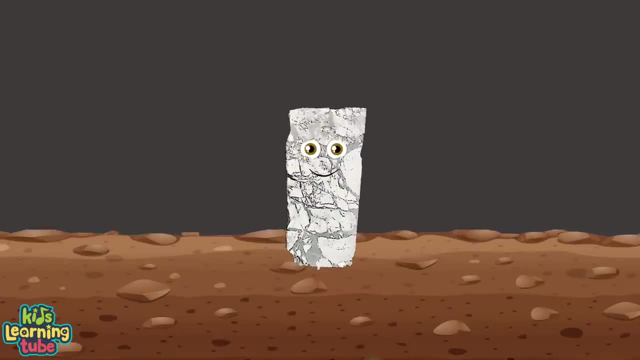 Here are some examples of the rock called sedimentary Limestone. sandstone and shale are three. you can now see I'm a type of rock called metamorphic. I am one of the main types of rock. to be more specific, Metamorphosis means to change and I'm transformed by heat and pressure from it. 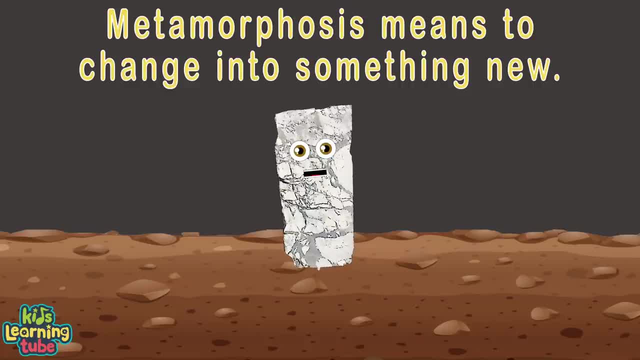 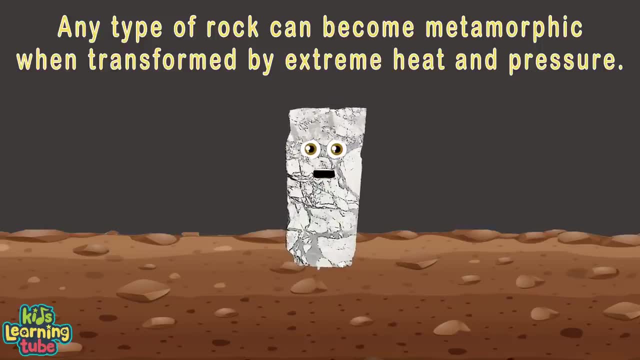 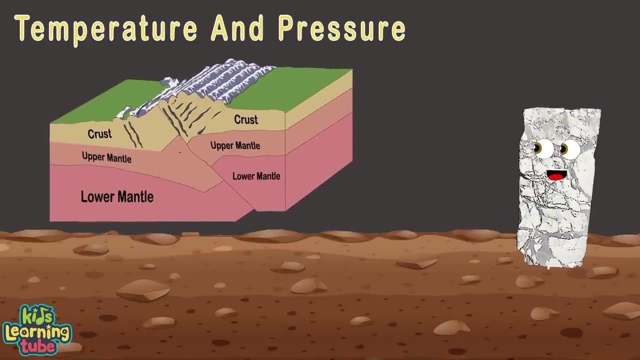 From existing rocks. here is more about me. Any type of rock can become metamorphic when transformed by extreme heat and pressure. like this, Metamorphic rocks form deep within the earth's crust Where temperatures and pressures are high. it's a must. 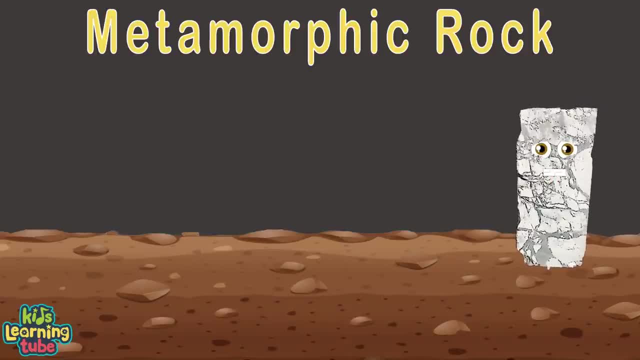 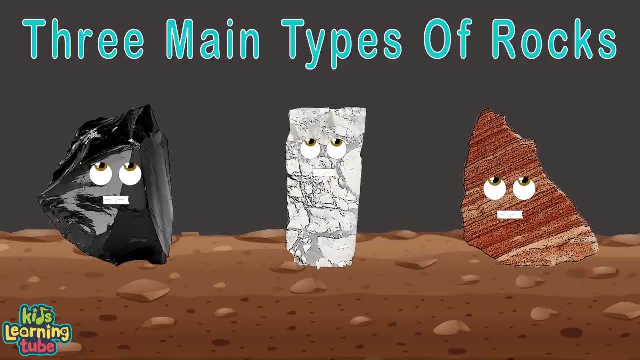 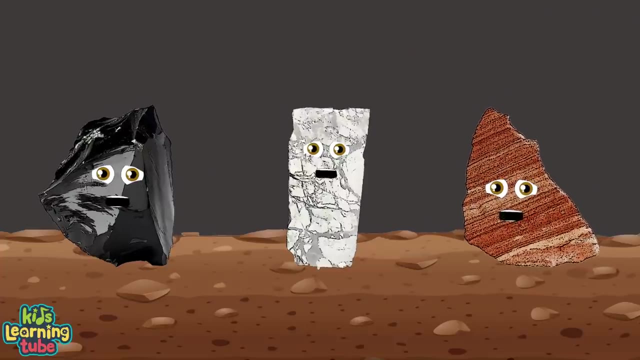 Here are some examples of metamorphic rock. I'll show lapis, lazuli, schist and beautiful marble. There are three kinds of rocks on earth you will see: Igneous, metamorphic and sedimentary. Our world is full of these rocks. on landing in the sea. 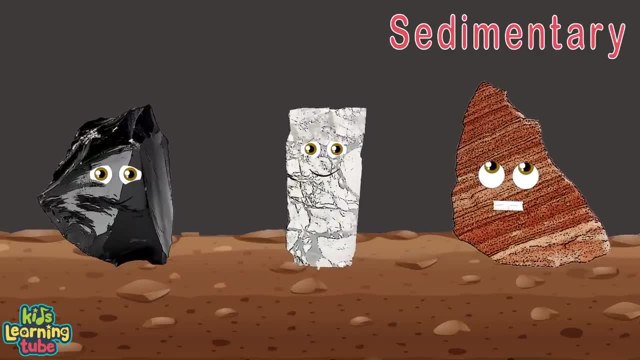 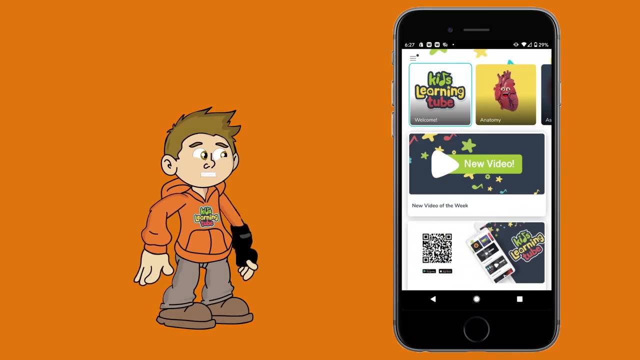 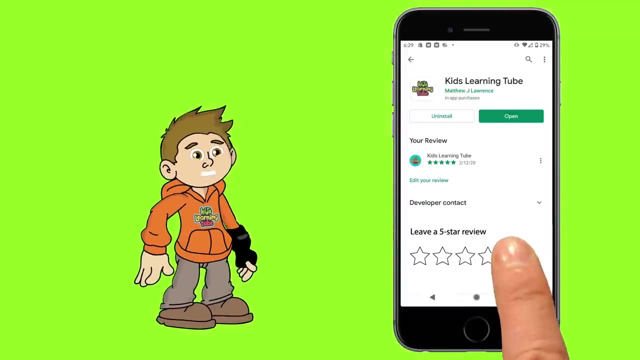 Igneous, metamorphic and sedimentary. Do you want a free monthly bonus video? Go. download the Kids Learning Tube app on iOS and Android to watch the weekly video and bonus video for free. today. Please leave us a 5-star review to show your support for Kids Learning Tube. 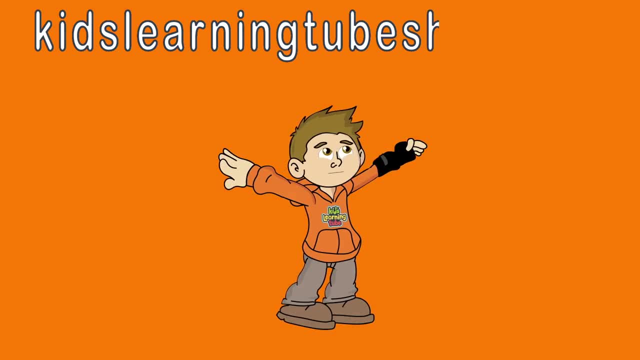 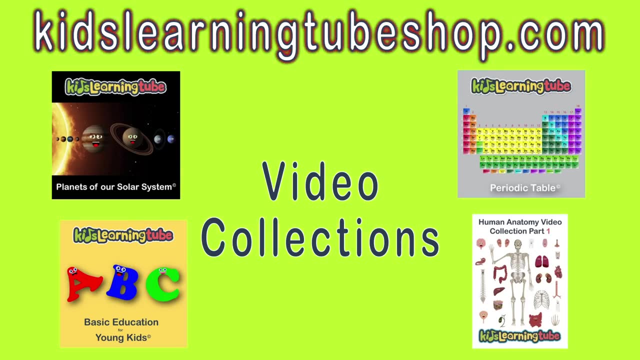 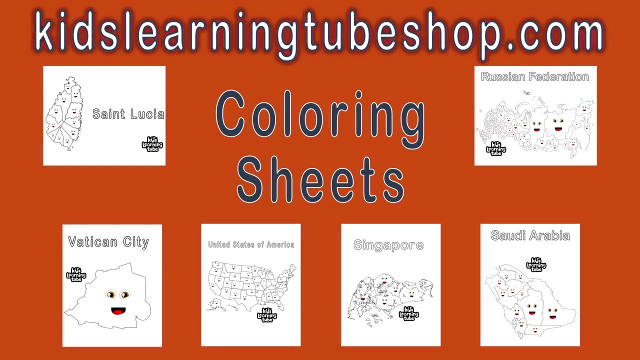 Find all your favorite merch at kidslearningtubeshopcom. You can get t-shirts, You can get throw blankets and pillowcases- Any video subject you want- from the Kids Learning Tube video collection. You can purchase your favorite music. You can get your favorite coloring sheet.